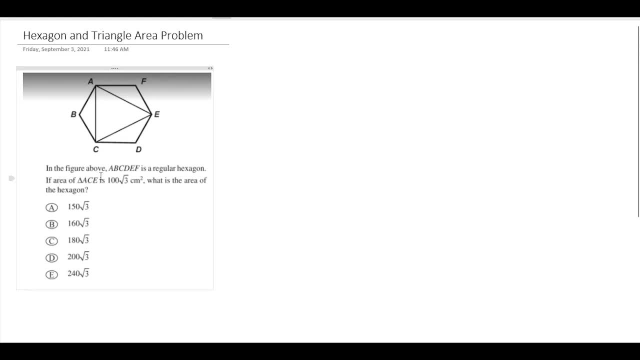 okay. so the problem is saying that in the figure above, abcdef is a regular hexagon. okay, abcdef, regular hexagon, that means all sides are equal. good, good, if the area of triangle abc is 100 under 3 centimeters square. so there is a triangle. it's kind of like inscribed inside of it a, c, e. 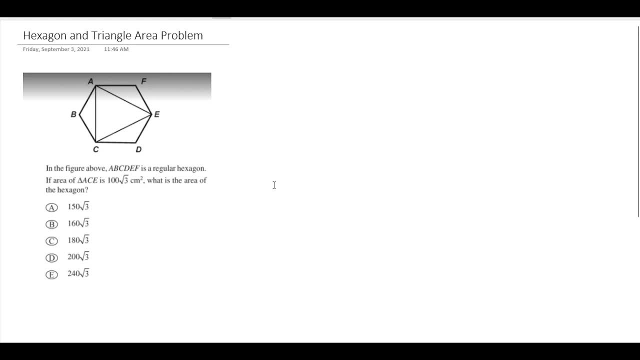 what is the area of the entire hexagon? okay, so, uh, honestly, i'm just gonna explain my thought process and how i approached it and how i was able to move to different approaches accordingly. so, first of all, the let's just draw this diagram really quick. so there is this hexagon. 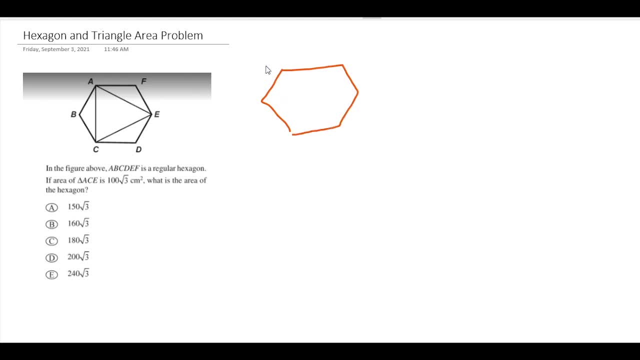 i'll try to be as accurate as possible and i have a, b, c, d and f, okay, and there's like a triangle over here and i know the area over here which is a hundred and root three, but what about the, its entire area? so to know the entire area of the 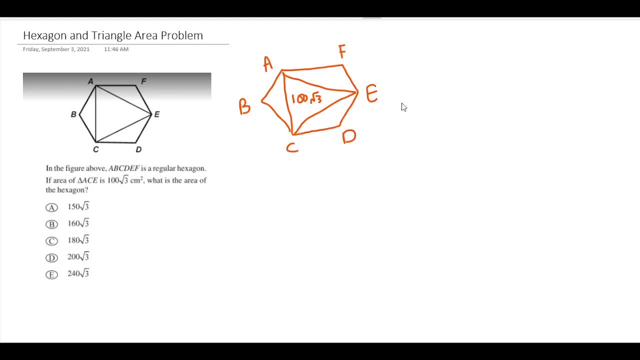 hexagon. first of all, there's like a quick uh, you know, a finite element technique in which basically what you do is, first of all you consider the hexagon and it's entirely, and then you kind of like, divide that into regular equilateral triangles and, if you have memorized your formulas, the area of the uh equilateral triangle. 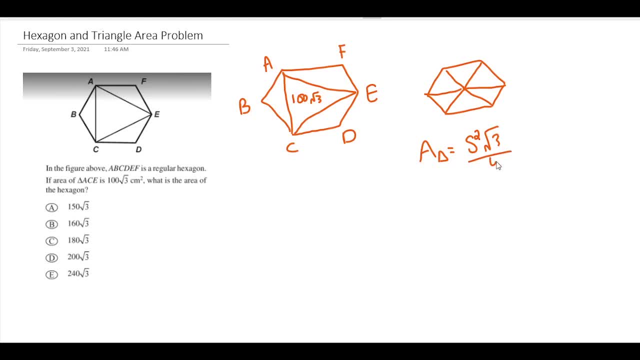 is side square under root, three by four. and if i want to find the area of the hexagon, what i'm just gonna do is, since there are one, two, three, four, five, six of these, uh, equilateral triangles, all i just need to do is take this, okay, and multiply it all with a six, okay, so i'm basically. 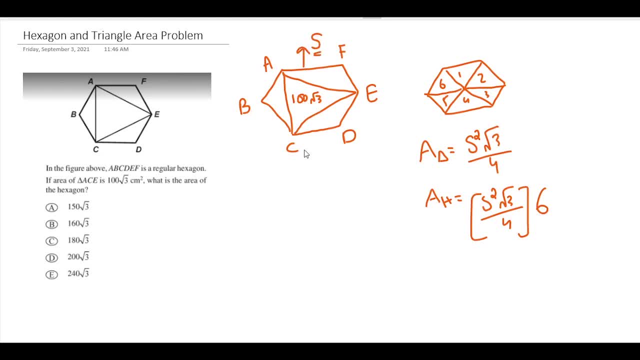 interested in the side, like that's my goal here. so now the question arises is: how do i do that? so first, what i did was okay. why don't i consider the sides and try to come up with the constraint so that if i know the size, i can ultimately get to this outer edge? so i was okay. why don't i consider? 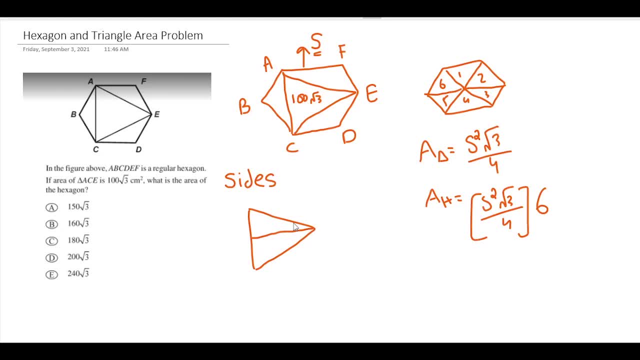 the side and the height. okay, and since i need the base and the height, so why don't i call this y and this x and this x? so the area is just going to be the base times the height, you half that, and then you get the area right which is given, uh, which is a hundred under three. 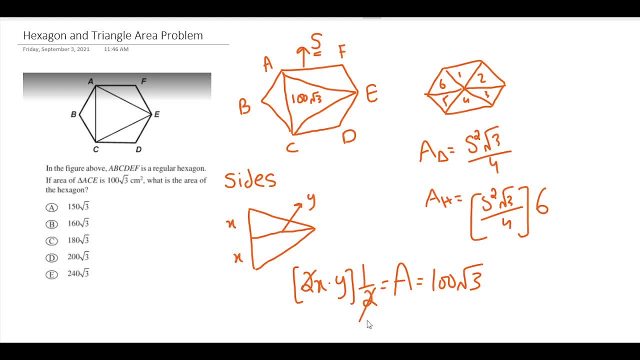 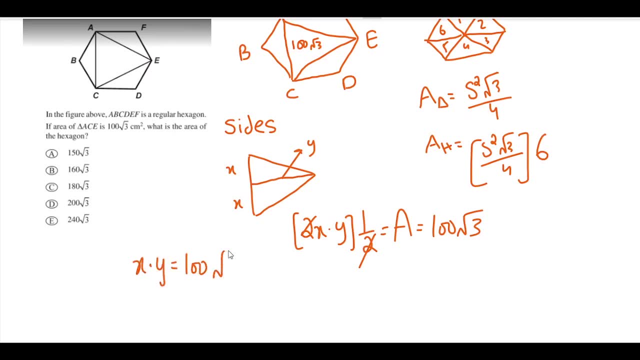 the problem over here is that, as soon as i just cancel my values out, now i have two variables with just one constraint, and there is no way that i can use these two variables to get to my s, which is basically my side, which i'm looking for right, right over here. 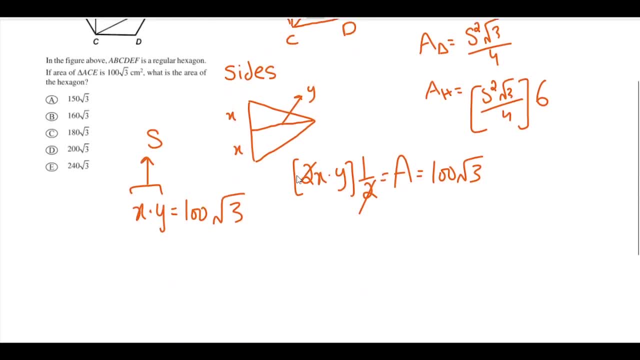 okay, let's just use green, because it's getting a lot of orange over here. so now i know for a fact that, hey man, sides are simply not helping me. probably what i need to do is go for the angles, okay, since we're in irregular polygons. so i was like, okay, why don't i? 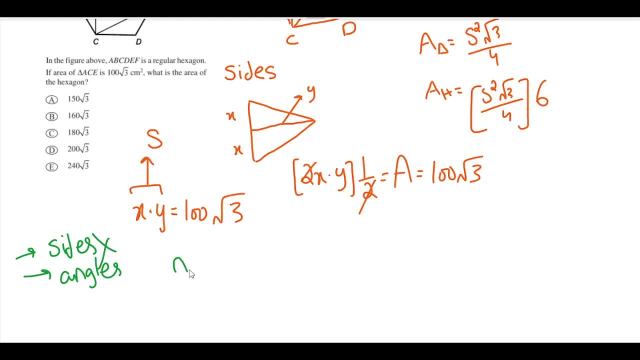 consider the angles. okay, so there this internal angle formula: n minus 2 times 180, and you divide that by 9, so since n over here is 6, if you simplify, you get 4, 180 times the 6, and what's this going to be? say 30. yeah, so every angle is 120. okay, internal angles, like all these angles. 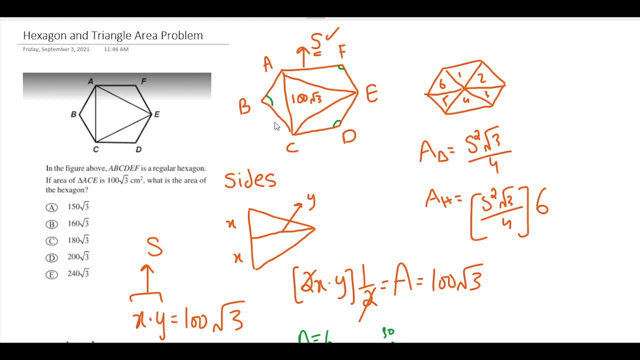 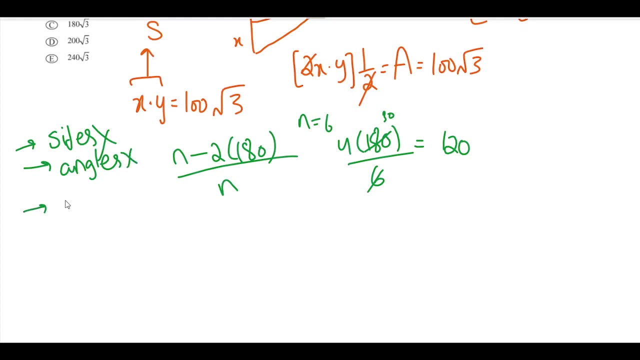 are 120. so far, so good, but again, is this giving me any type of relationship so that eventually, i can get to my s value? not exactly, so. now i'm just going to cancel this approach as well and go to my uh, even though it sounds a bit more engineering type, but this method is known as the 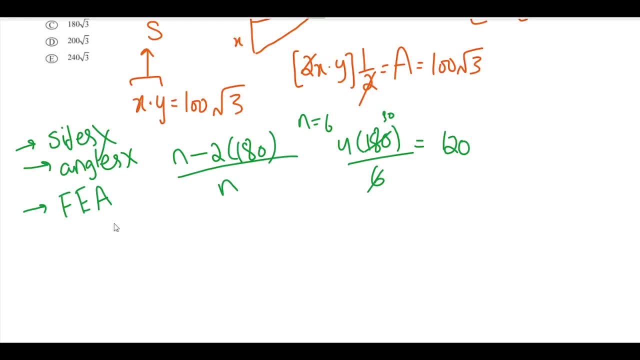 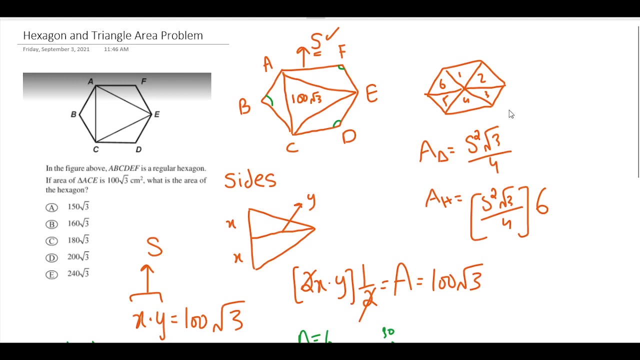 finite element analysis. so basically, what you're trying to do is you're trying to consider the given value of the angle and you're trying to break them apart into similar units and try to come up with the relation from there. so if you come back over here, i did this, like i've already done this, like i've taken a small unit which 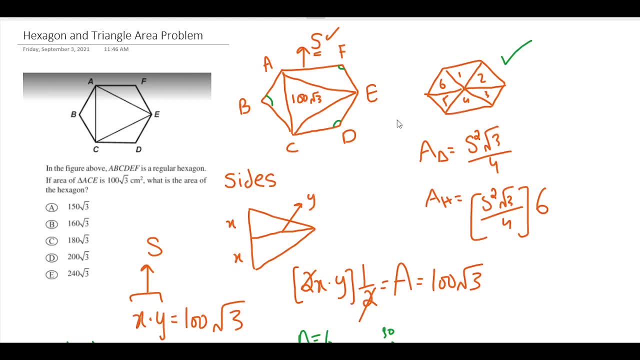 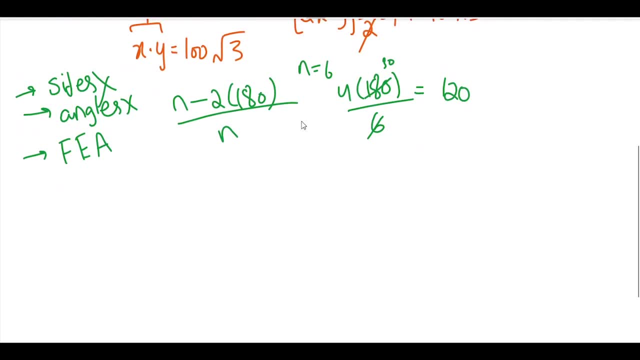 represents the entire hexagon. and now the question arises: what about the triangle? i've done with the hexagon, but what about my triangle? can i do something with this? so let's try to do that, okay, right over here. so this is, let's say, this is my triangle. 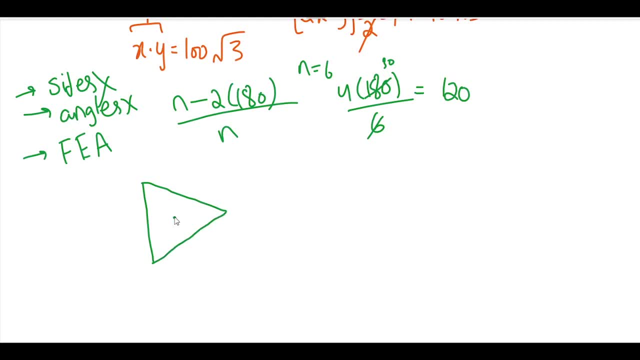 okay, and if i divide it from the center, same thing. i'm just going to try to make it as much clean as possible, okay. so the overall angle is 360, and if i divide 360 with a 3, i'm getting 120. so there's 120 over here, 120 over here, 120 over here. and now what i'm going to do is i'm 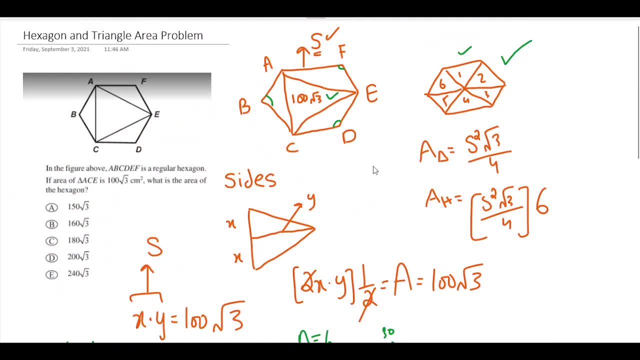 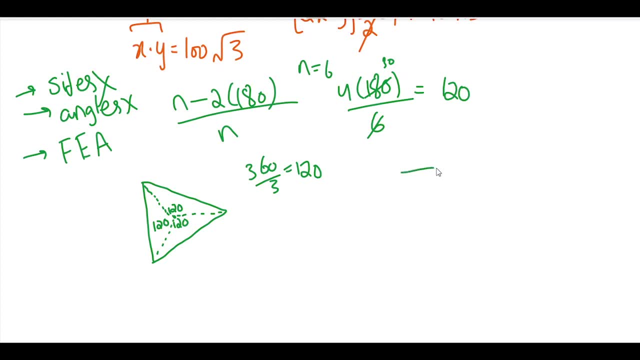 just going to use these elements and this element over here and try to see if i can find a relationship. okay, that's all what i'm doing. so if i make this diagram a little big this time, just so that i can address everything out, this is this hexagon. yeah, looks pretty neat. and now what i'm 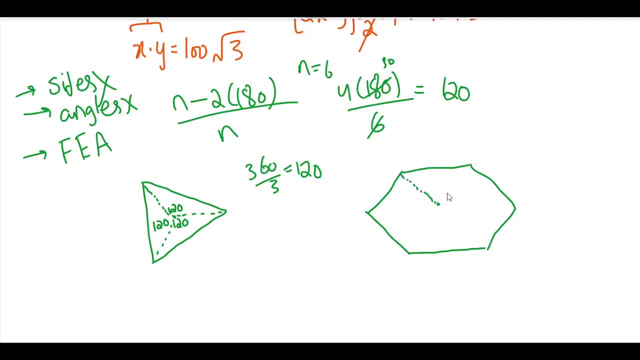 going to do is take this and take this and draw it over here. now, these are the same lines, all which have 120, 120, 120, okay, and here's the crazy thing, all these angles are also 120. we just proved that right. 120 and all of these sides s s s are all equal. here's things, but here's, here is where things. 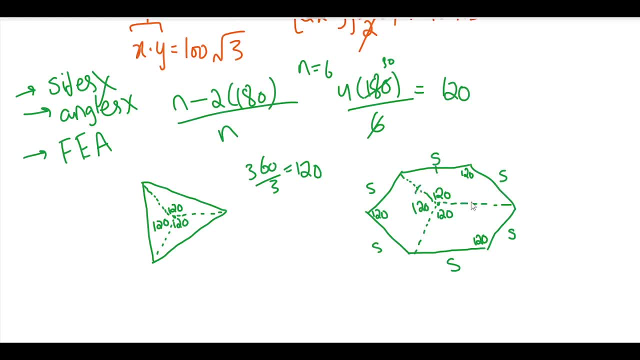 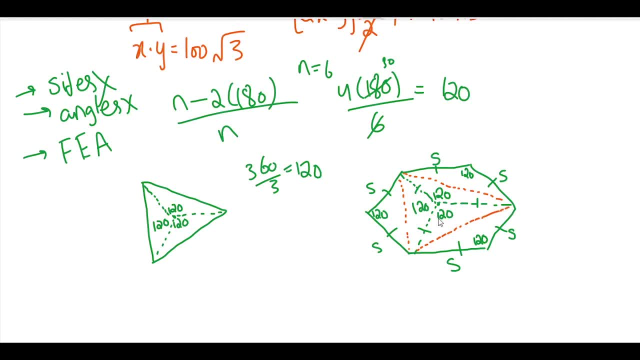 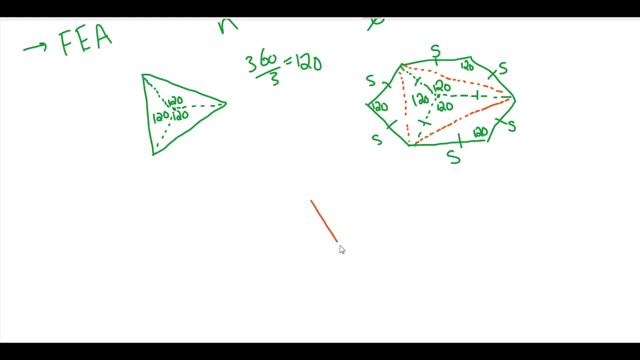 things get really interesting. now. i have literally similar- in fact equal- triangles. how, like, if i drop it, let me just draw it over here. this is s and this is 120 over here, and right on top of it, this is s and this is s and i have 120 over here, and let's call this side to be i don't know q. okay. 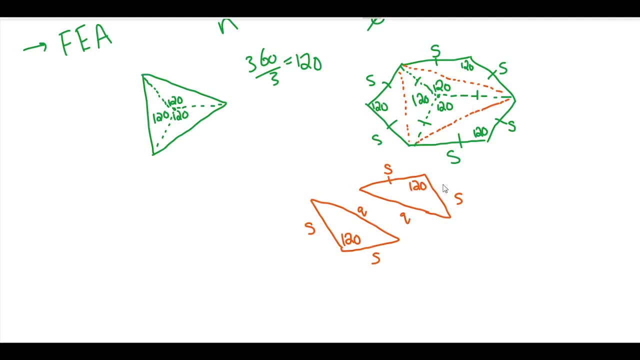 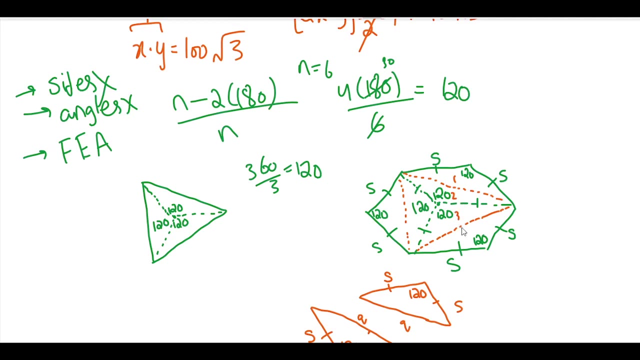 so you can see all sides are similar. okay, the respective sides are similar, they both have similar angle and therefore we are basically going to have a similar angle and therefore we are basically looking at one, two, three, four, five and six exactly same triangles. okay, it's more of like 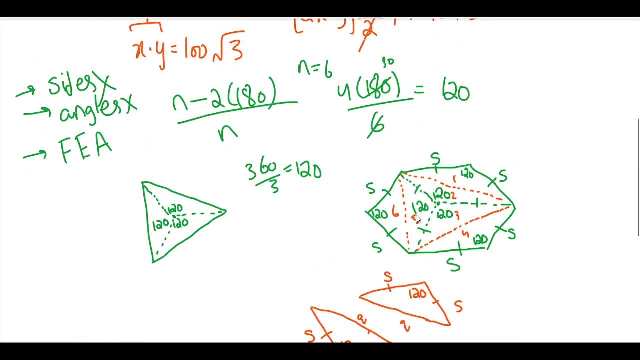 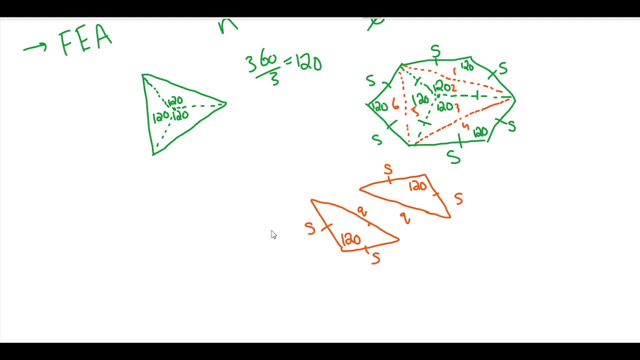 what we did with the hexagon, but when we combined the triangular and hexagon, we're basically looking at six similar triangles. are you following so far, or do you have any questions? yes, yes, you're following, okay. okay, so now here's the thing. so, when we are combining three triangles, 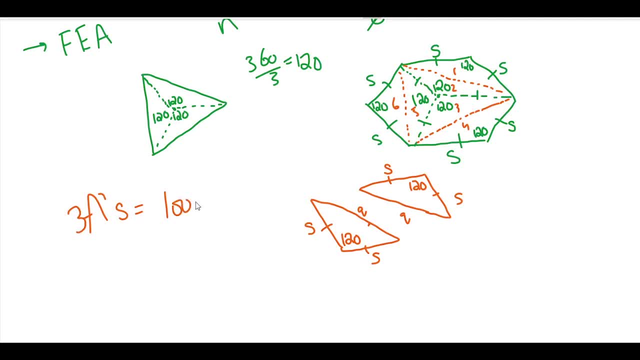 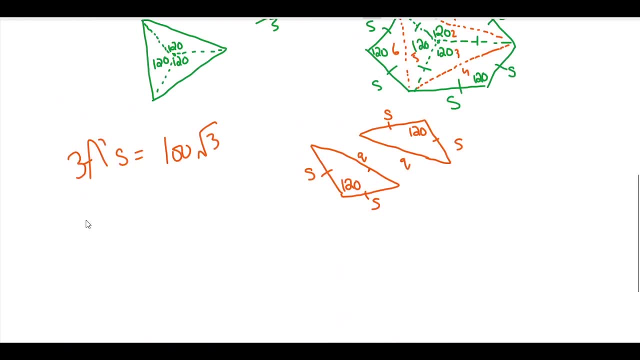 their area is hundred under root three. let me just confirm. let me just go back up. yeah, so what is going to be for just one triangle area? well, that's just going to be hundred over three under root three and since we're interested in hexagon area, which is basically similar, six. 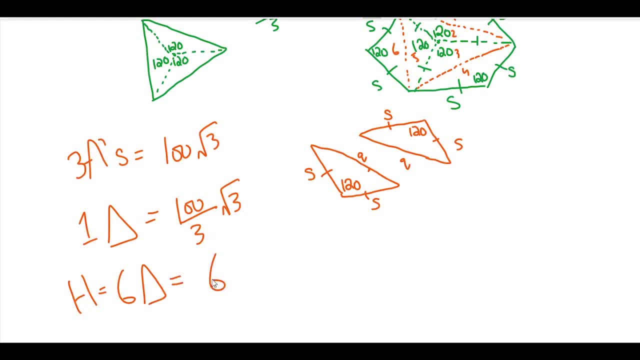 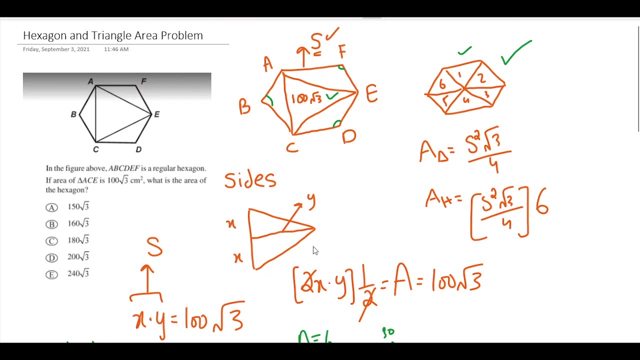 triangles, exactly same triangles. all i need to do is just multiply this with three, and if i do a little bit of simplification, i'm getting 200 under root three. and if i come back up, uh, yeah. answer must be the following: so far, yeah, yeah, okay. so is that it, or you want to discuss? 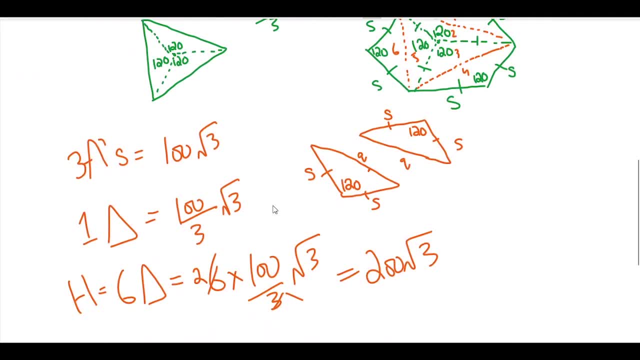 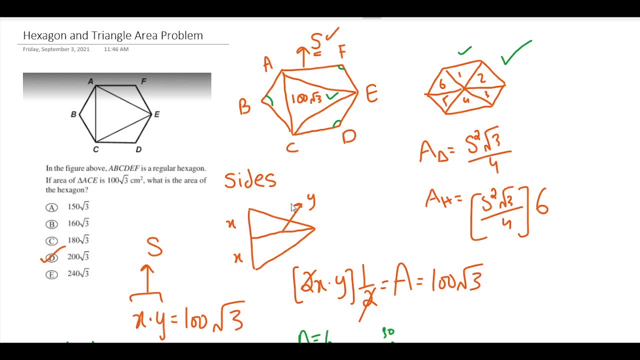 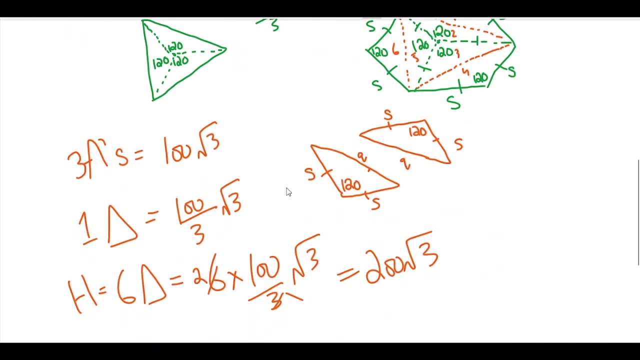 anything else as well. no, no, no, it's very clear. no, okay, thank you so much, man, have a great day. yeah, thanks a lot, abd, thanks a lot and abd, uh, what do you suggest um to practice uh, verbal, that means, could you provide any tips for verbal? 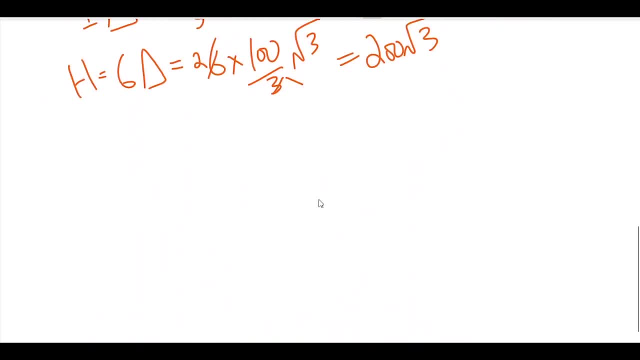 okay, so verbal, uh, i would have to say that you know, uh, ets like ets is unmatchable, like i have literally tried other third-party materials but they are nowhere close to ets because when it comes to the logic and when it comes to you know a 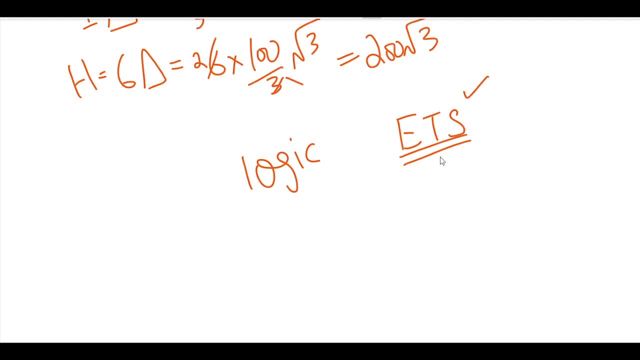 like i said, you can use a lot of books, but you're going to be very interested in the like the more consistent arguments for every single option. ets is the king, so i would suggest that you, uh like ets has a lot of books, man, i don't like. how many books have you like it has? like the old? 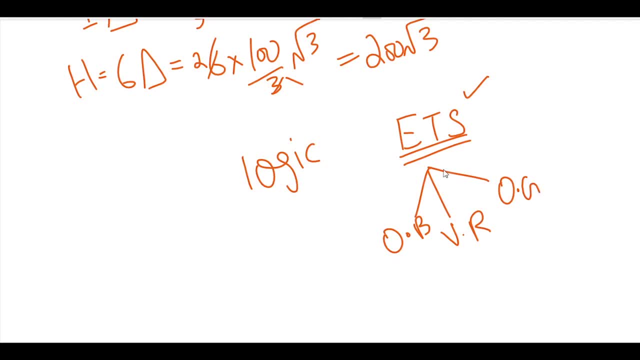 book, old book. it has the verbal reasoning book. it has the official guide. it has- i don't know, two practice test books, practice test books. then there are two mock tests on free, on the ets. i mean, they have a lot of material, man, so i would suggest you and they. 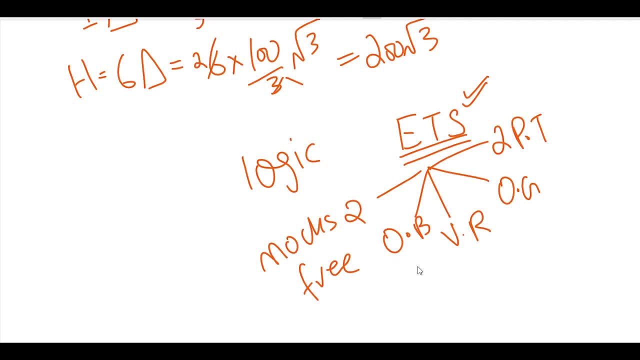 also have a big book, something, yeah, old book, the big book. you know, this is the big book, yeah. so i would suggest that you use ets only and don't go here and there, because their content is absolutely amazing and spot on at beginning how we need to start every day like. 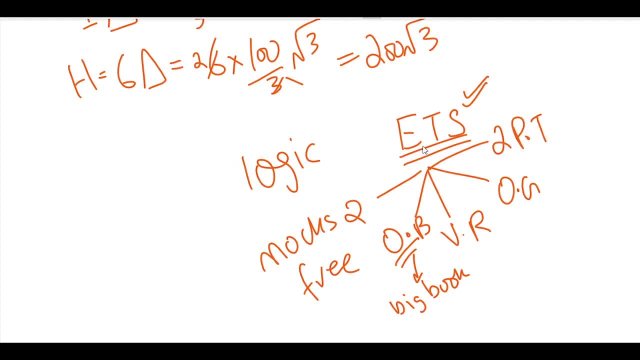 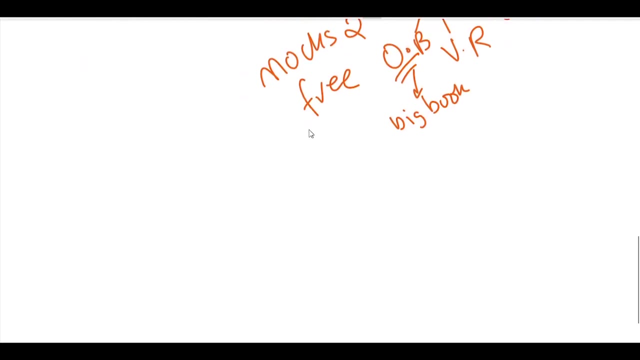 um, for example, when i'm taking sentence equivalence, how should i figure out the logic? how should i figure out the logic? okay, so at beginning i don't know anything right, i don't know the synonyms and all, so how we need to eliminate, so any tips? so, okay, so here's the thing. 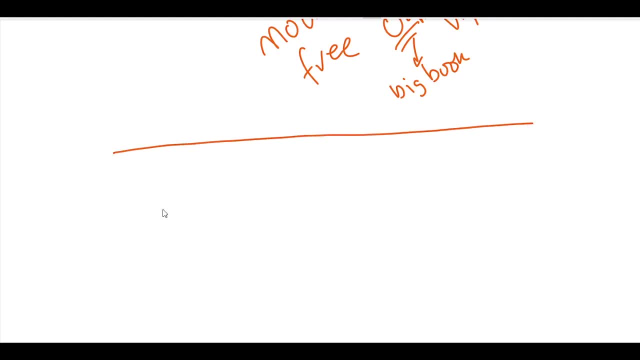 so, initially, what you need to be doing is, let's say, this is the entire sentence, and then there's a paragraph. so you're not going to get everything right, and so this is the way you need to be doing it, okay. so your goal should be to guess a word, okay, which is as close to the correct answer. 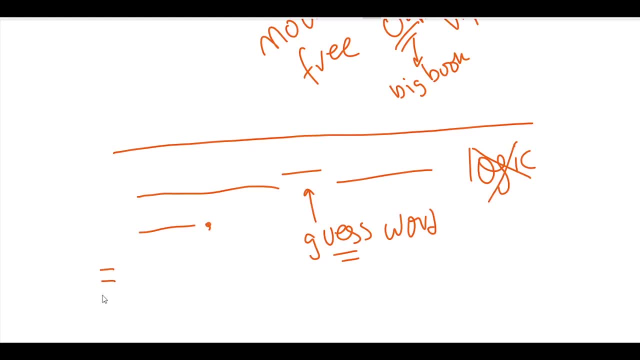 because if your guess is wrong, that means you cannot understand the logic. you follow me. don't worry about the vocab just yet. okay, don't worry about the vocab work on that, because at the end of the day, there is no escaping from vocab. if you are basically looking at a 155 plus,